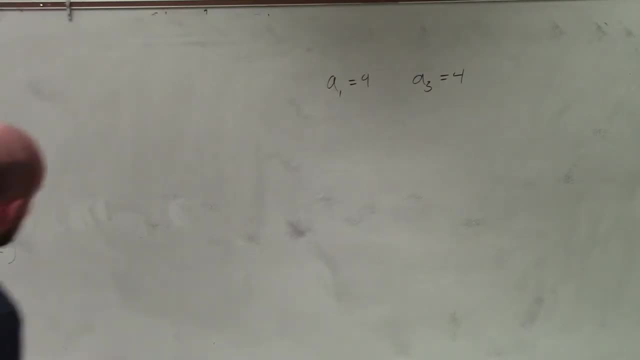 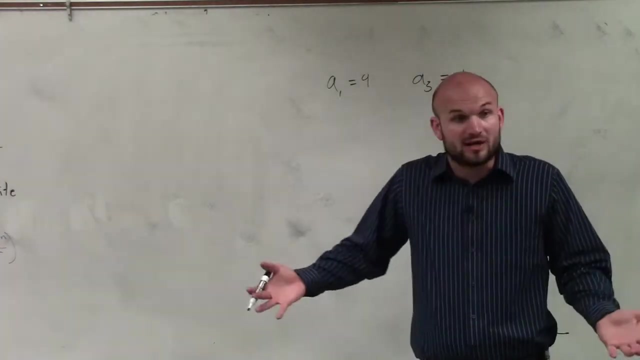 So in this case again, what they're asking us to do is be able to identify what They want us to identify: the first five turns of the geometric sequence. So to do that, we need to identify what r is correct. Yep, okay. 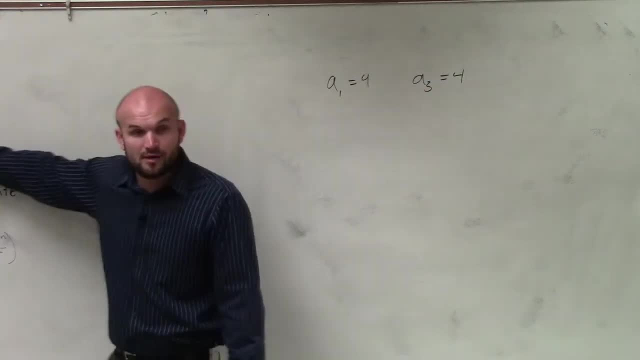 So to identify r, we need to go back to our rule. Well, it's very basic. I want you to make sure you have this and understand how to identify it. So our rule for a geometric sequence. you guys should hopefully remember the one for the arithmetic. 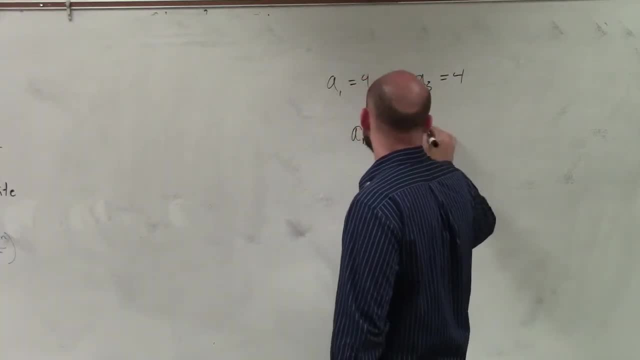 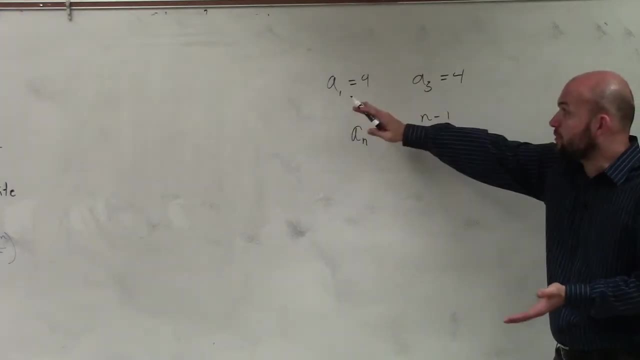 the geometric is: a sub n equals a sub 1 times r raised to the n minus 1,. all right. Now again we don't know what r is, so let's plug in the values. Now we know what a sub 1 is, which is 9, and we can say a sub 3 is going to represent our n. 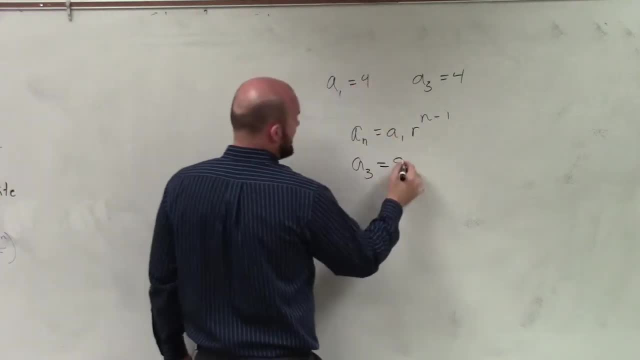 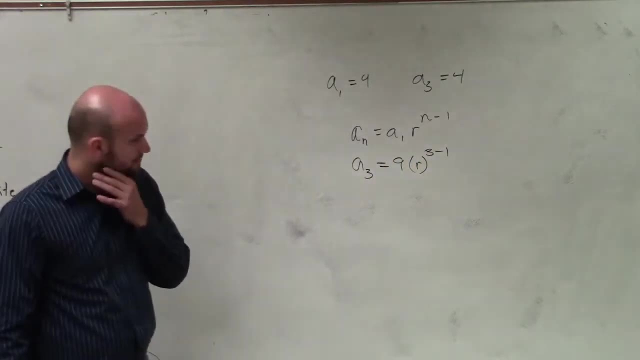 So therefore, we have: a sub 3 equals a sub 1, which is 9, times r, which we do not know, raised to the n, which is 3, minus 1, correct, Yeah, a sub 3 is 4.. 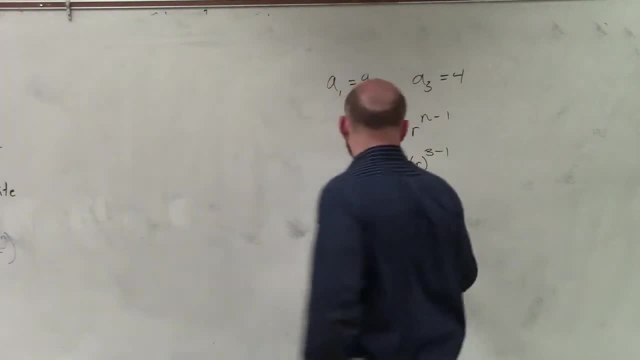 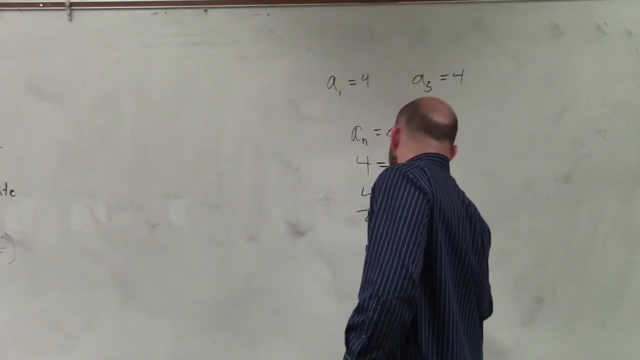 So now let's go and solve for r. 3 minus 1 is 2, so I have 4 equals 9, times r squared. divide by 9.. 4 ninths equals r squared. To solve for r, I take the square root: r equals 2 thirds. 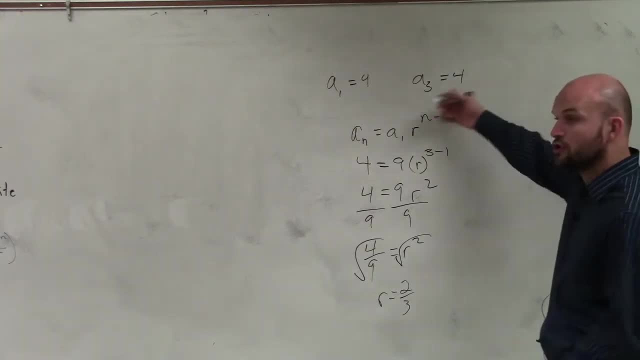 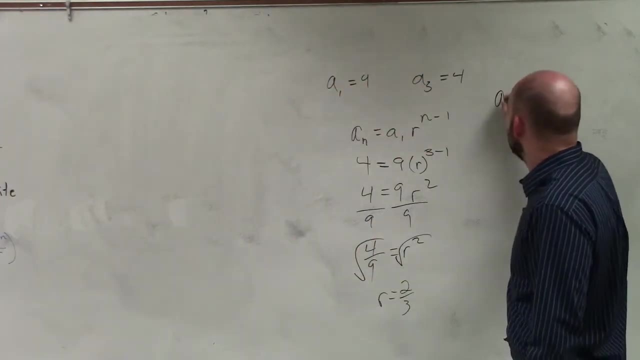 Now, again, I need to identify the first three terms. So I'm going to go back to my formula, because this is much easier to use the formula than it's always going to be to find the common ratio to me sometimes. So I have a sub 1, which I know is 9.. 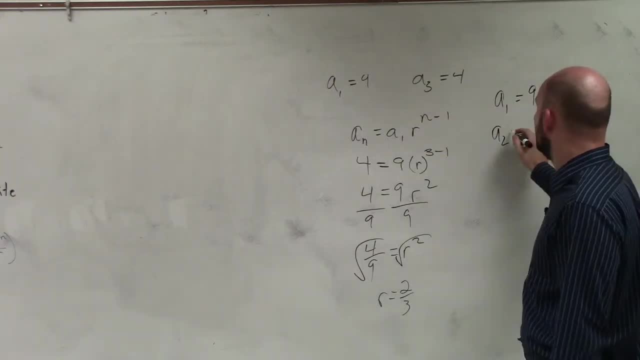 A sub 2, let's use the formula, It's going to be a sub 1, which is 9, times r, which is 2 thirds times 2 minus 1.. Well, 2 minus 1,, ladies and gentlemen, is 1.. 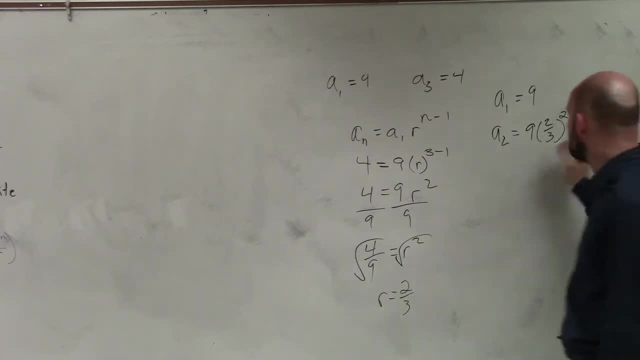 So therefore it's 2 thirds times 9,, which is 18 over 3,, which is 6.. Let's do a sub 3.. 9 times 2 thirds over 3 minus 1.. Does everybody see how I just plug in for a sub 3??